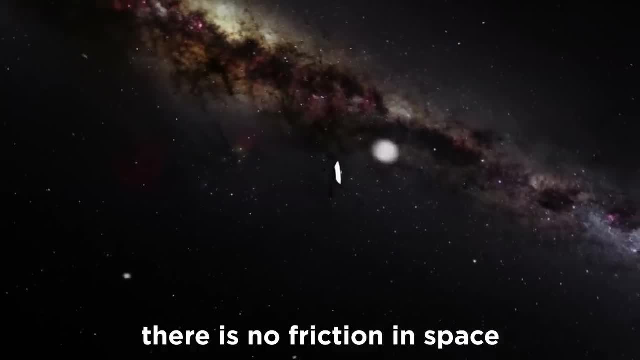 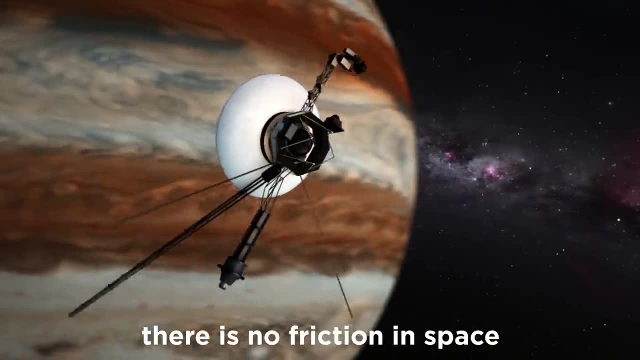 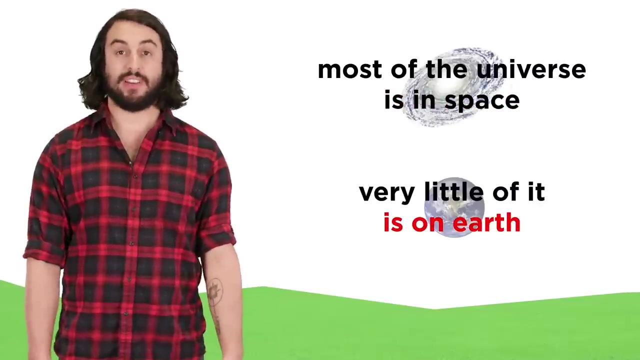 This is the kind of motion that can be seen in the vacuum of space: Stars and planets and asteroids and satellites. these objects have roughly constant velocity and they never stop moving. As it happens, most of the universe is in space and very little of it is on earth. so we should 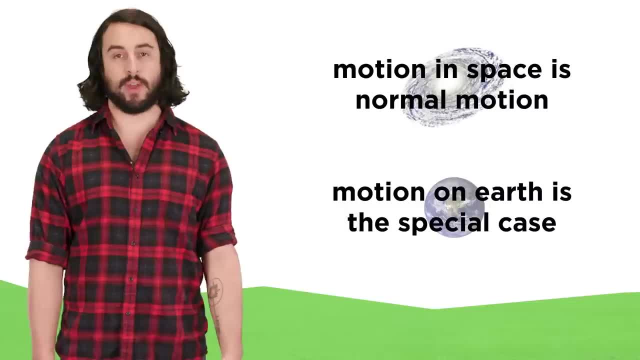 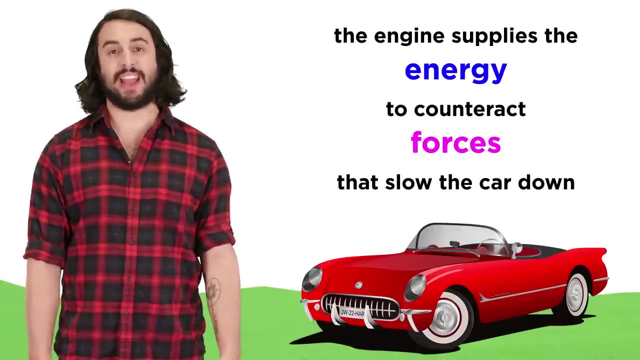 consider motion in space where there is no friction and no wind resistance to be normal motion. It is motion within earth's atmosphere. that is the special case where objects are subjected to a variety of variables. This is why a car needs an engine that is always running, because there is resistance. 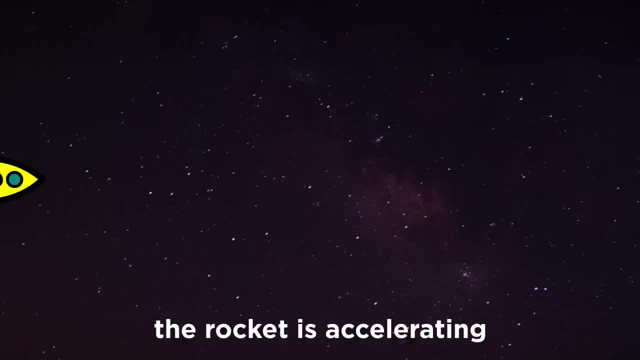 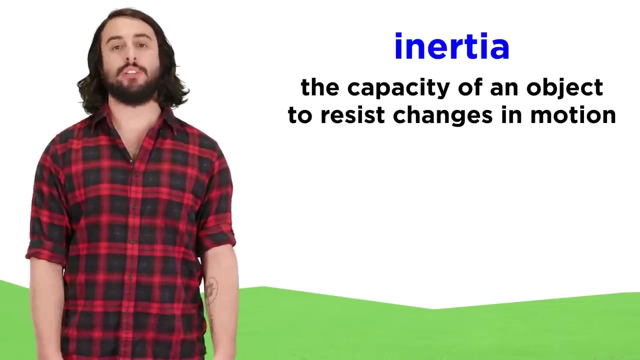 from the atmosphere and friction with the road. But a spaceship can just accelerate to a certain velocity and then turn the engine off and it will cruise at that final velocity without end. The capacity of an object to resist changes in motion is called its inertia. 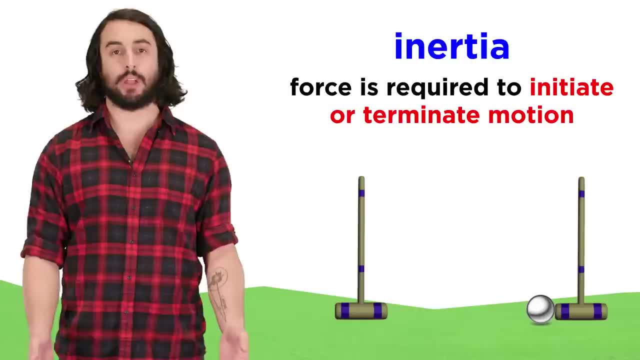 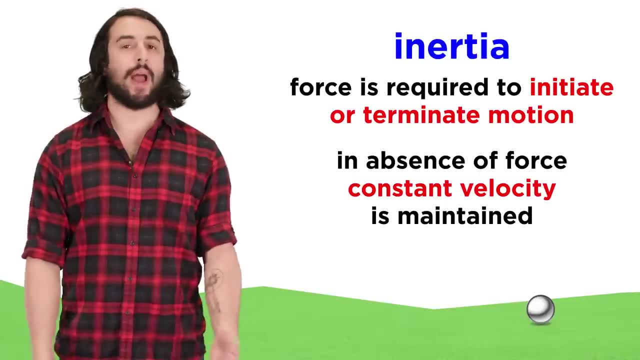 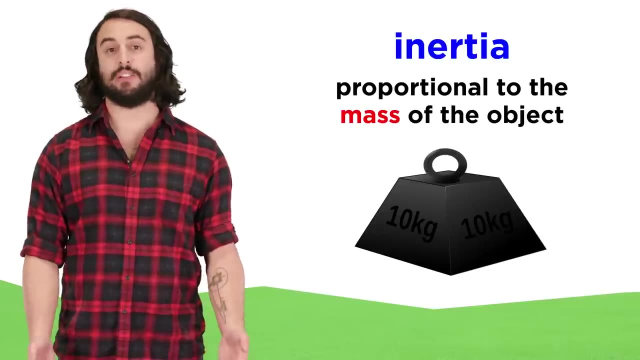 Force must be applied to get an object moving and again to slow it down to a stop Only. motion with constant velocity, including zero velocity, requires no application of force. An object will have some amount of inertia that is proportional to its mass. a scalar. 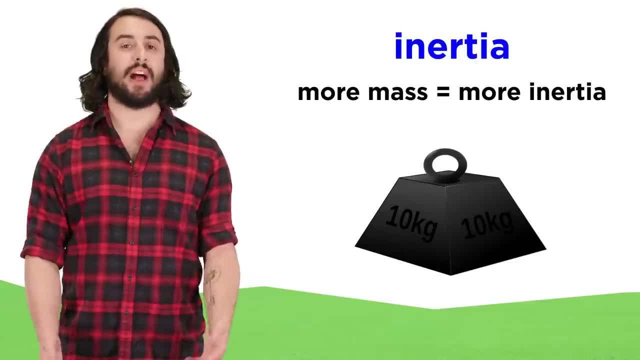 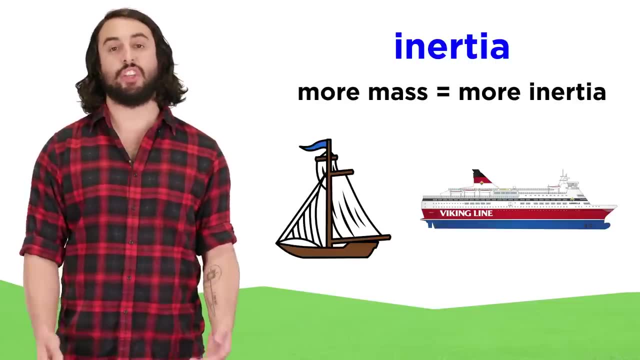 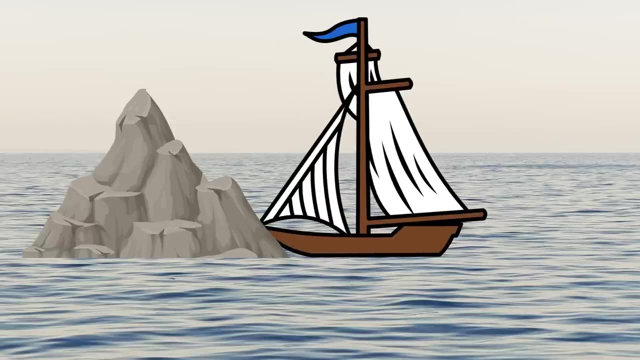 value measured in ki. More massive objects have greater inertia or greater resistance to motion. Think of a tiny sailboat versus a huge luxury cruise ship. A strong gust of wind is enough to get the sailboat going, and if it hits a rock, it. 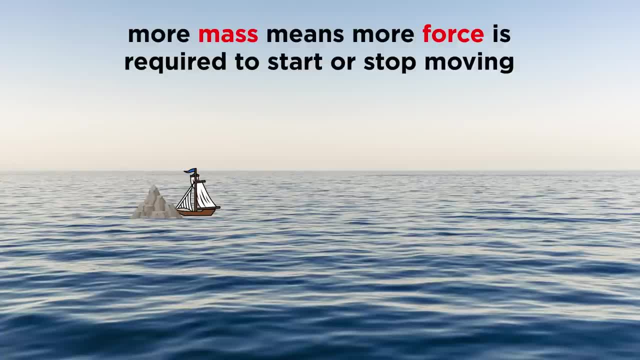 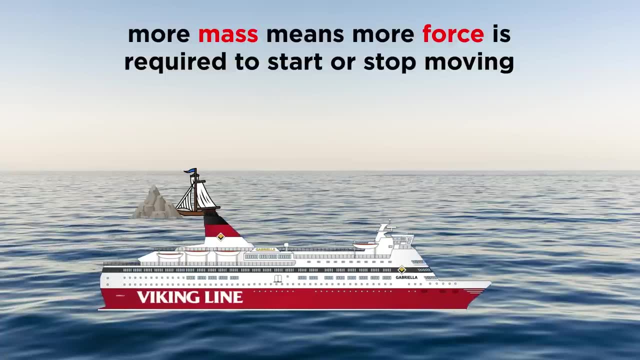 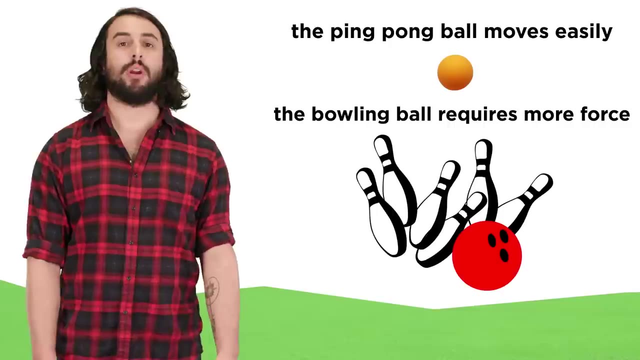 will stop on impact, But the cruise ship needs huge engines to accelerate from rest. A lot of force is needed to get it going and a lot of force is needed to get it to stop. Similarly, it is easy to set a ping pong ball in motion. just give it a flick. 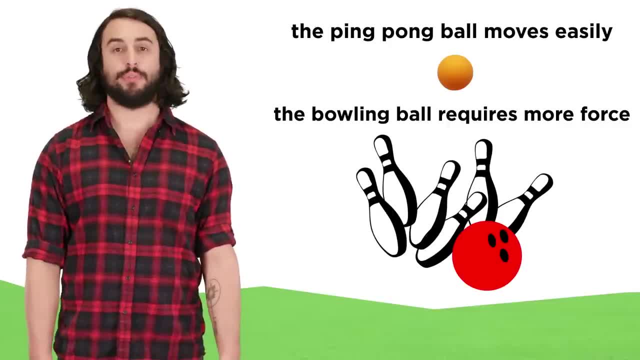 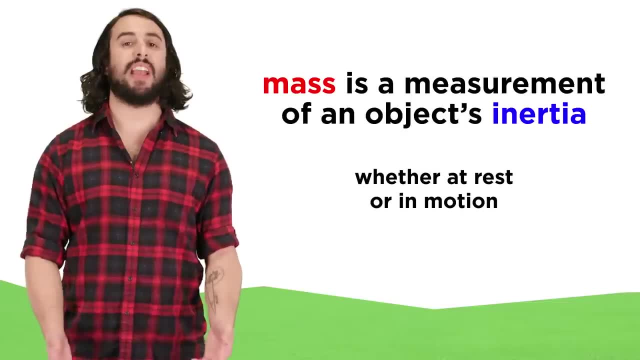 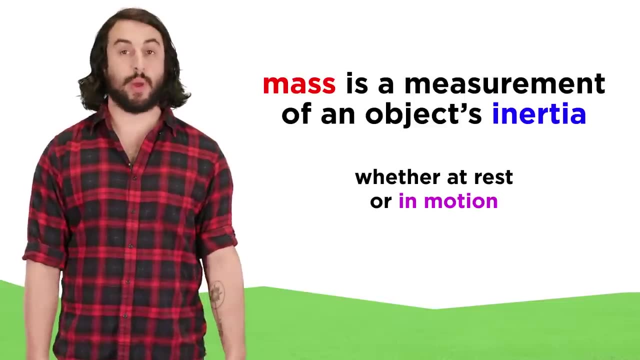 But a bowling ball will need quite a bit more force, and more force to stop as well as any bowling pin will tell you. In this way, mass is essentially a quantitative measure of an object's inertia. As we said, this applies to objects that are already in motion as well. 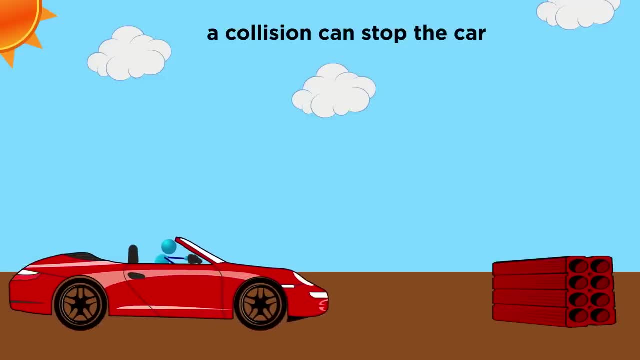 If you get into a car accident, the force of impact will stop the car, but your inertia dictates that your body is in motion. If you get into a car accident, the force of impact will stop the car, but your body will tend to continue moving.